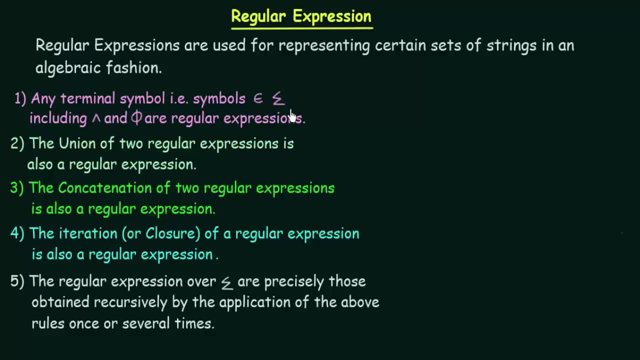 Any terminal symbol, ie symbols that belong to sigma, including the empty and the null symbol, are regular expressions. So till now we have seen many symbols like a, b, c and so on, which we use for representing the inputs and outputs. 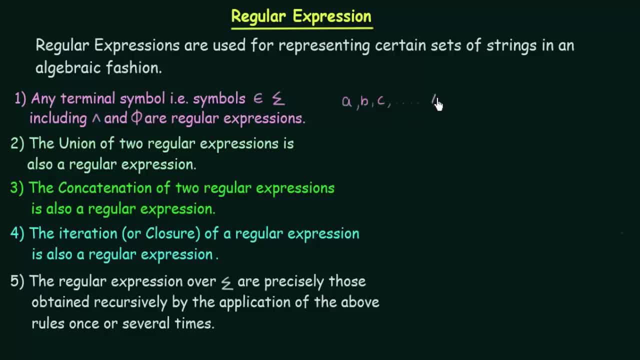 So all these symbols known as terminal symbols, including the empty and the null symbols, are all regular. So I need 1 terminal symbol. 1 terminal symbol means that a two station or average signal, A and b, have two station. A and b must serve as the union of a virtual problem to a regular signal. 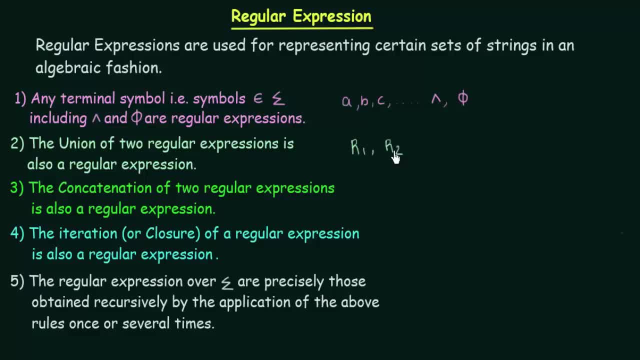 Because once again we know the union of the two regular expressions are also regular expressions. So because once again we are given firstそして a, b and b are Uber is just regular. our second terminal symbol must look like this in order to represent a regular expression: 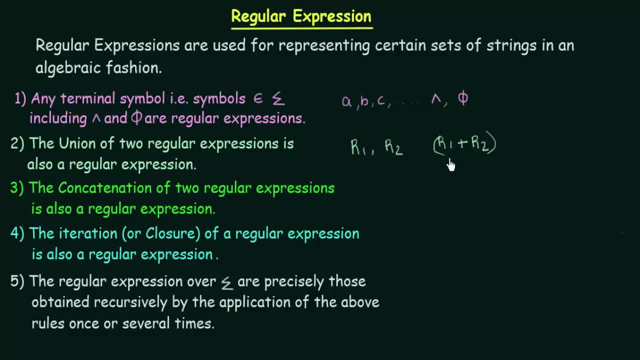 File date Line kto. R1 and R2 are regular, then their union will also be regular, Alright. so let's see the third point: The concatenation of two regular expressions is also a regular expression. So let's say, we again have two regular expressions, R1 and R2.. 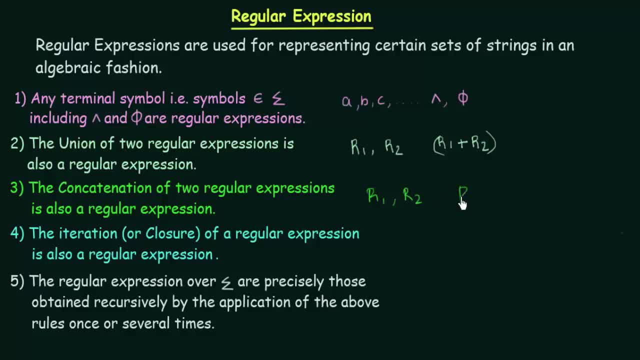 Then the concatenation of these two regular expressions, which is represented by R1, R2, or you can even put a dot in between them, So this will also be a regular expression. So if we have two regular expressions, their concatenation will always be a regular expression. 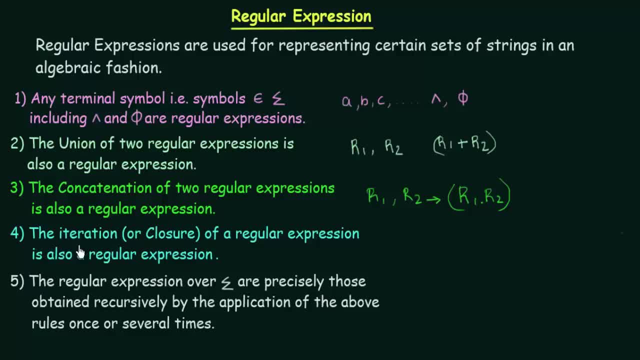 Alright, so let's come to the fourth point. The iteration or closure of a regular expression is also a regular expression. So if we have a regular expression, let's say R, and then the closure of R, which is represented by R star, will also be a regular expression. 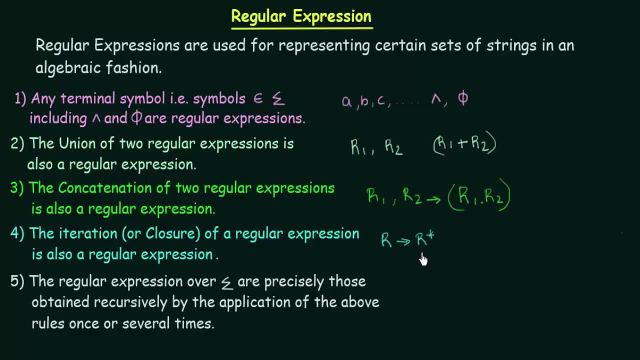 So what is this closure? I have already mentioned and discussed about this closure in one of our previous lectures, But let me just repeat it again. Suppose we have a symbol A, and then the closure of A, represented by A star, will be everything that you can form using this A. 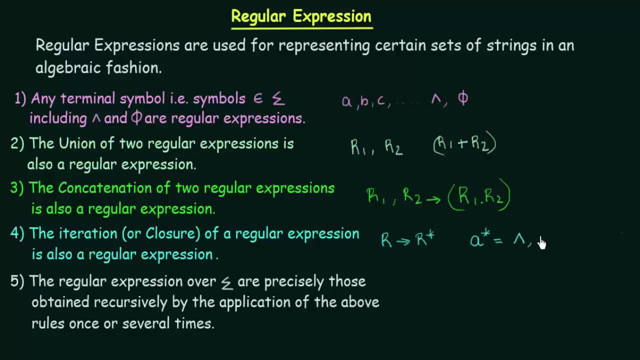 So it includes the empty symbol as well as A, and then AA, AAA And so on, Everything that you can form using this A. it will be an infinite set. So that is the closure of A. So if A is a regular expression, then its closure will also be a regular expression.